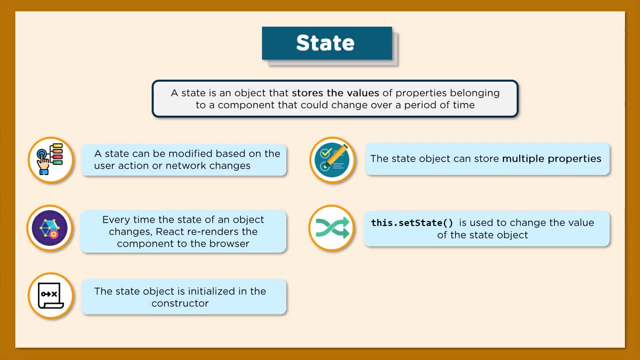 A state can also store multiple properties. A method called setState is used to update the value of the state object. Now this function performs a shallow merge on the new and the previous state. Conventionally, a shallow merge ensures that the previous state values are overwritten by the new state values. 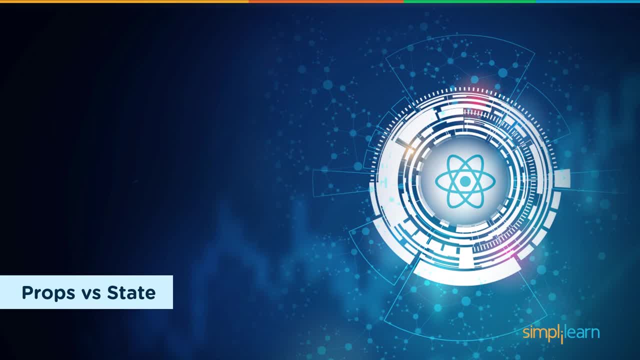 Moving on. In our previous video, we learned about props, And although props and state dictate and control the behaviour of a component, they have significant differences. So let's go ahead and draw a comparison between the two. Firstly, props in a component are used to pass data and event handlers to its 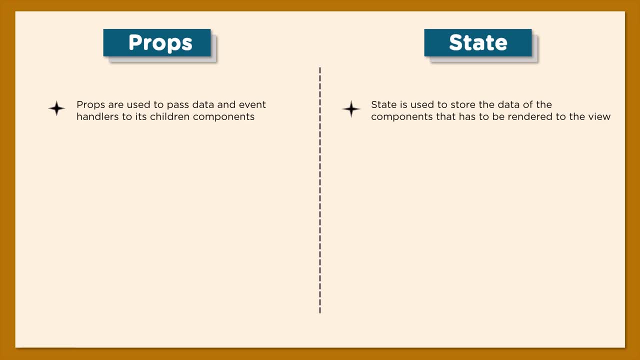 children, while state, on the other hand, is used to store the data that has to be rendered on the webpage. Props are immutable: Once set by the parent, they cannot be changed. State holds volatile data and can be changed over time. Props can be used in functional and class components, while state is restricted to class. 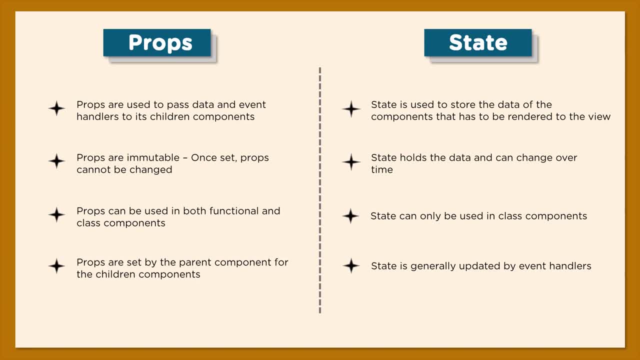 components, Props are set by the parent component, while a state is generally updated by event handlers. Now that we've learnt all about state, let's go ahead and build an application to see the working of state. Alright, so in my code editor- that is vs code- I've created my application. say state. 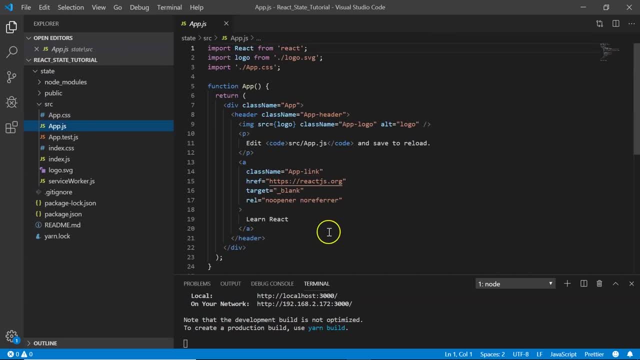 And here in my source folder, I have my appjs file. Now, here I'm going to get rid of all the unnecessary code that I'm not going to be using. Also, I suggest you go through the react installation on windows video to help you get started with. 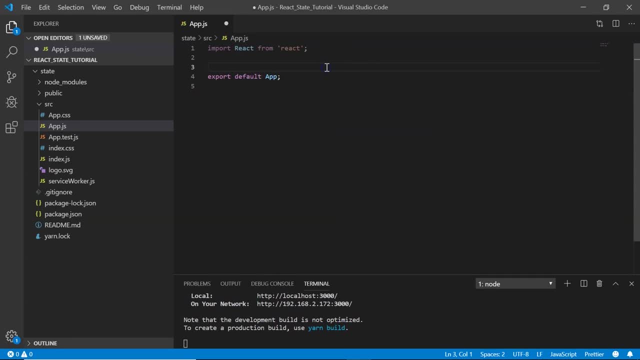 creating your first application. So let's create our class component, say, class app extends reactcomponent, and inside I have a render. Let's find a method that returns an HTML tag. Let's display a message: welcome. Let's follow the JSX conventions and enclose all the HTML tags within the div tag. 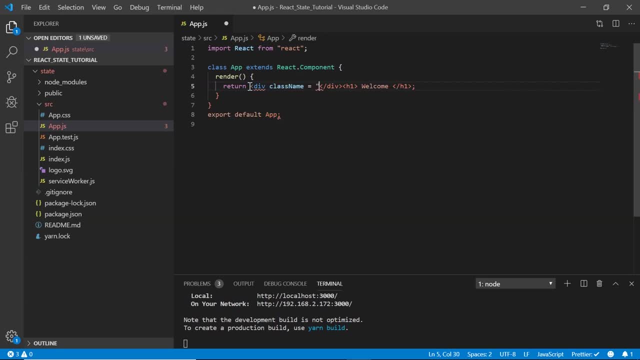 So I say div className equals app. We also have to import the appcss file. import appcss So we save it. and if you look at the browser we have welcome. Now let's beautify our code To do that. let's add some styling. 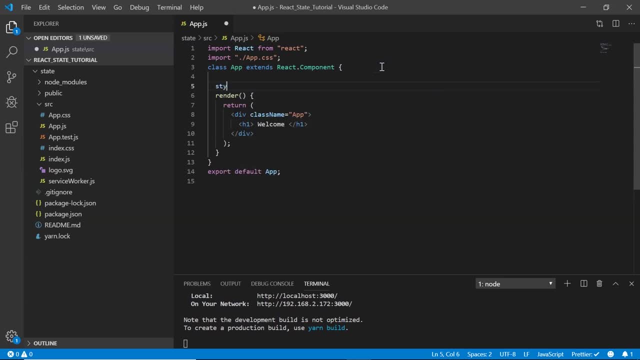 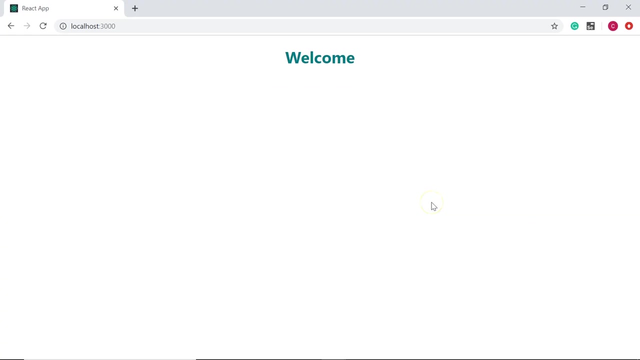 So here in my appjs class component I say styles equals and I say font style and I set it to say bold, and I say color, say teal, And here in my h1 tag I say style equals thisstyles. So let me save it and if we look at the browser now, we have welcome in teal and it's bold. 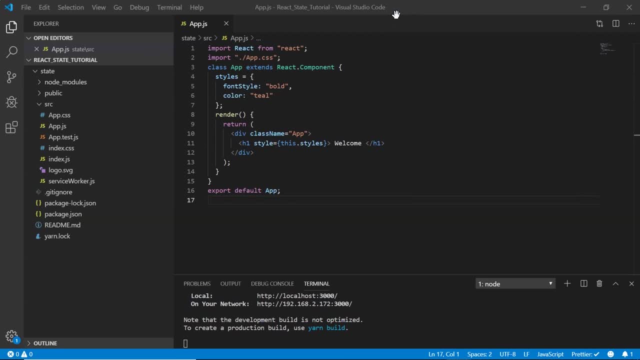 So let's add some style, And here in my h1 tag, I say style equals thisstyles. And here we add some style And I say style equals thisstyles And it's bold. Now let's go ahead and create a class component to understand state. 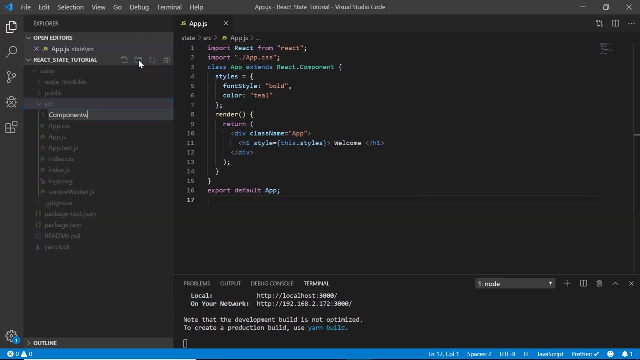 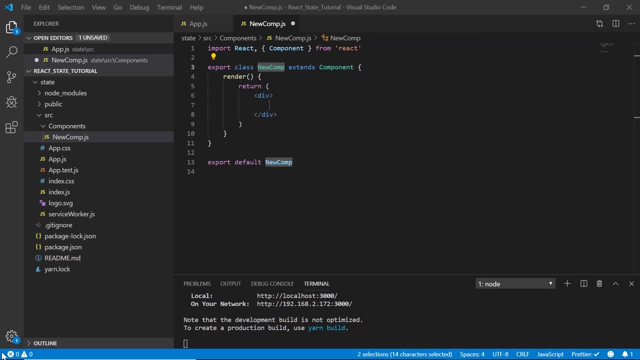 So first I create a folder and I call it components, and inside this folder I create a class component and I call it new compjs, And I use the snippet rce to create the class component. To give you an insight into what we're doing today, we'll display a message asking the: 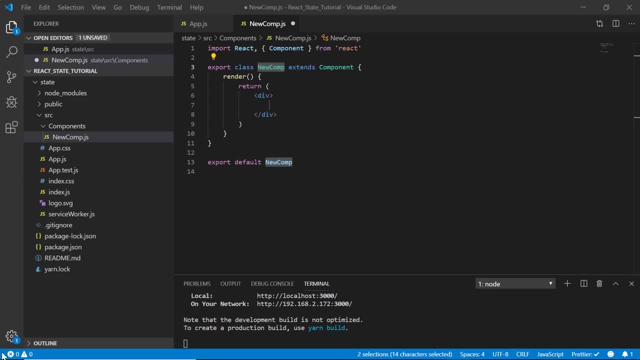 user to subscribe, to simply learn. Once the user clicks on the subscribe button, instruct them to click on the bell icon and, finally, we display a thank you message. now, to do all of this, we're going to make use of state and, as mentioned earlier, we initialize the state. object: 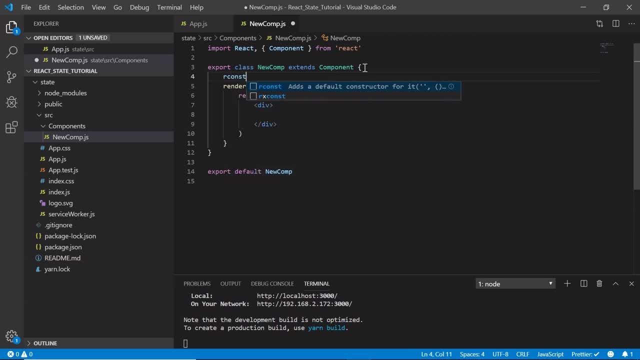 in a constructor. so let's use the snippet our const to create a constructor. now, in the state object, we initialize a property, let's call it message and we display a message saying subscribe. to simply learn, let's save it. and here in our render method, let's say class name. 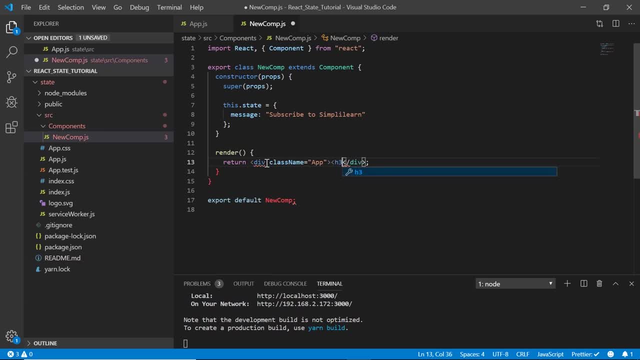 equals app and let's create an h3 tag and within the tag i displayed the message. so i say this dot state dot message. let's save it and now let's import it in our appjs component so i'll get rid of export here and here i say: 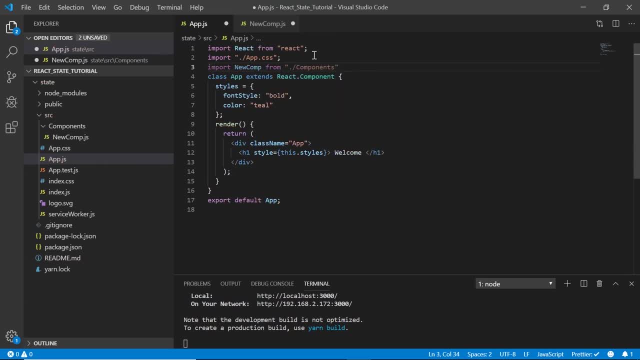 import new comp from components and new comp and let's define it here and say new. so we save it and look at the browser: it says subscribe, to simply learn. all right, again, to make our code look more presentable, let's add in styles. so i'll just copy the same styles that i've added here and i put: 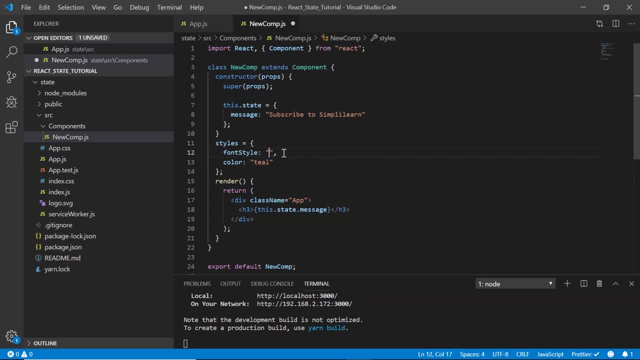 them here and instead of bold i make it italic and i change the color to say purple. and again in my h3 tab and i change the color to say marriage purple today. so i paste it here and i close it out and it's nice and if you are changing the color inside the string, the next time you do it. 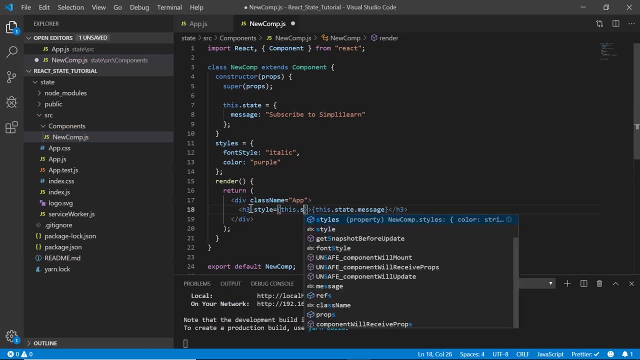 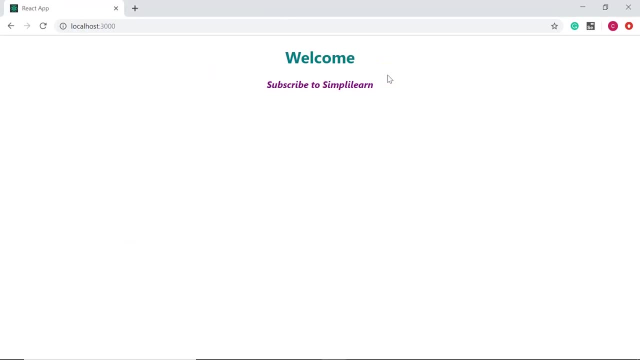 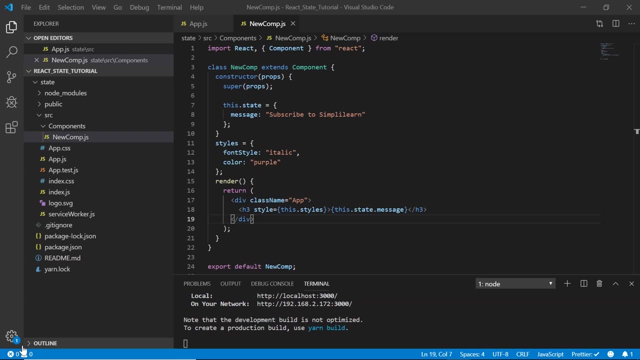 I define style and initialize it with thisstyles, so let me save it. and now, if you look at the browser, it's in italic and it's in purple. okay, so moving ahead, let's create a button that reads subscribe, and once the user clicks on it, the button should read subscribed and the message displayed above should: 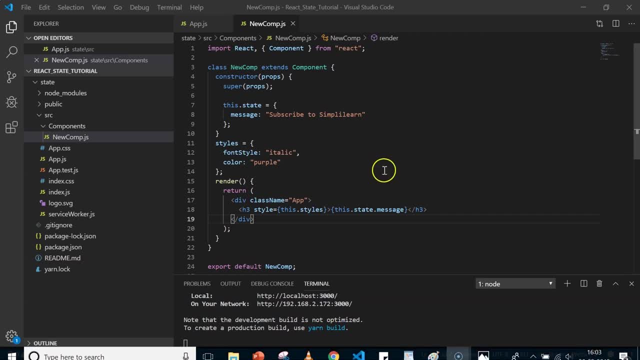 instruct the user to click on the bell icon. to do that, let's first create a button. the message that I want the button to read is subscribe. however, this message gets changed once the user clicks on the button. so instead of explicitly mentioning subscribe, here I create a prop. I. 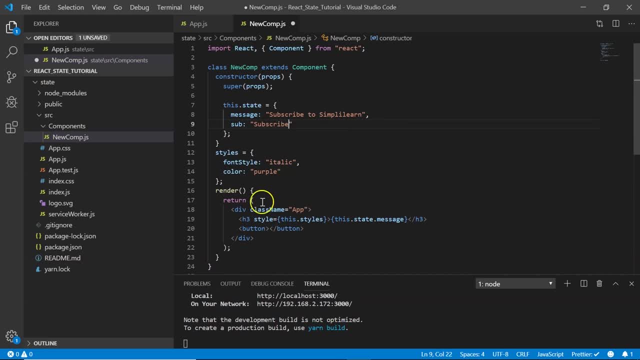 say sub and I say subscribe. here and back in my render method I say this: dot state, dot sub. so let's save it. and if you look at the browser now, you have a button which displays the message subscribe now. once the user clicks on the button, the message displayed should change to click on the bell icon to never. 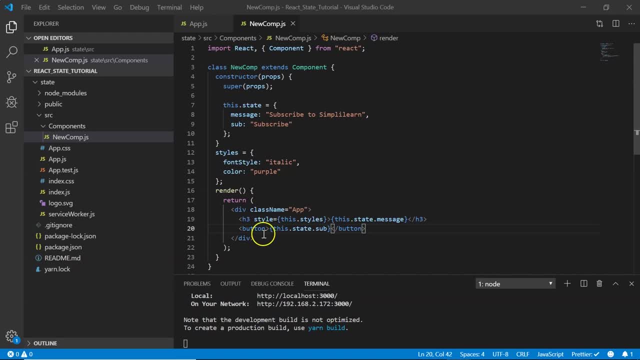 miss an update. So let's create an event handler for that. So here, button onClick, I call another method and let's call the method buttonChange. Okay, so this method should update the state and change the message and sub values. To do that we make use of a setState method. 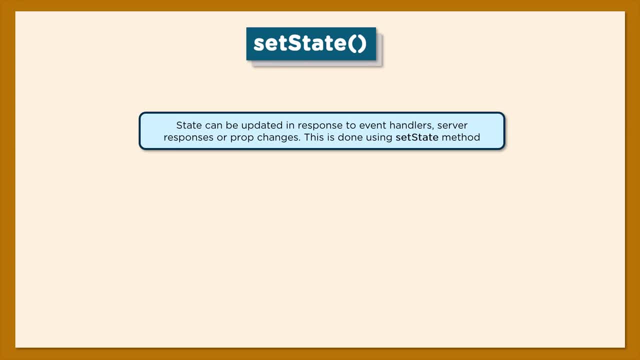 Now a state can be updated in response to event handlers, server responses or prop changes. Now all the updation can be done using the setState method. This is the general syntax used by the method. We'll have a look at this further in the demo. 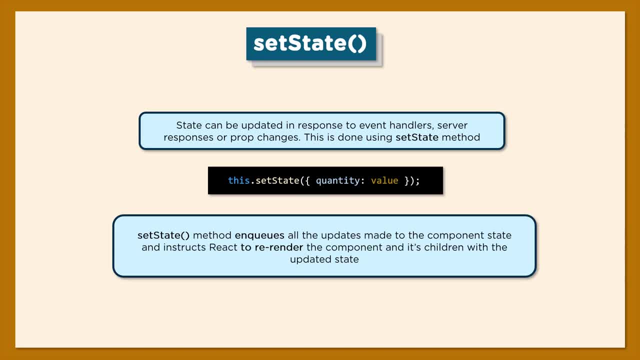 Now the setState method conventionally enqueues all the updates made to the component's state and instructs React to re-render the component and its children with the updated state. Now let's go back to our code editor and look at the working of this method. 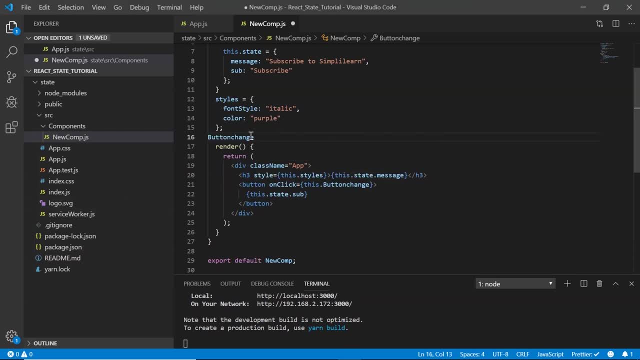 Now, here I defined the arrow function, buttonChange. If you are not familiar with arrow functions, I suggest you read up on them. This is the general syntax, And here I say this: ThissetState, And inside I change my message to hit the bell icon to never miss an update. 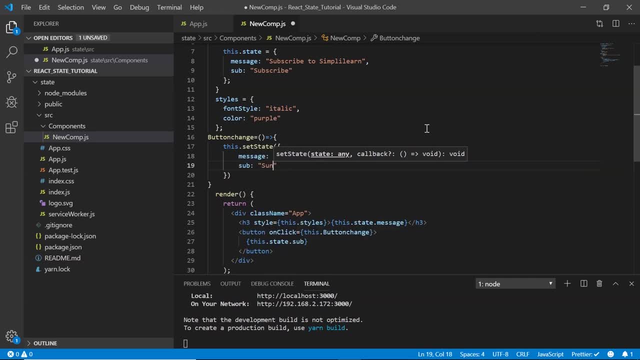 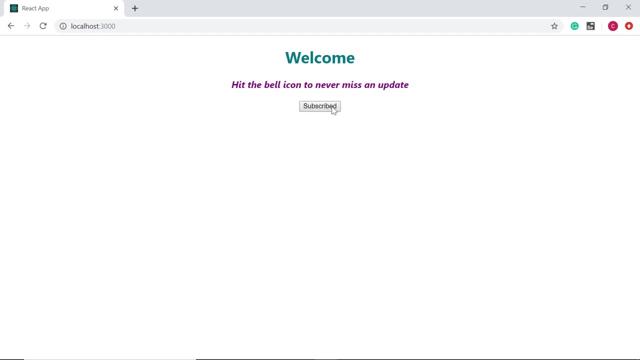 And my sub value changes to subscribed. Let's save this. And now, if you look at the browser, when we click on the subscribe button, the message changes to hit the bell icon to never miss an update. So, moving ahead, let's use a bell icon so that the user can click on it. 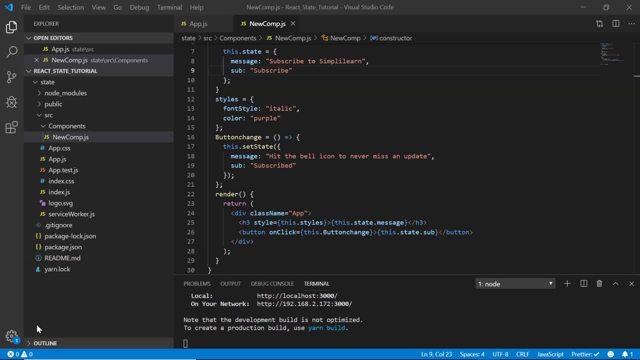 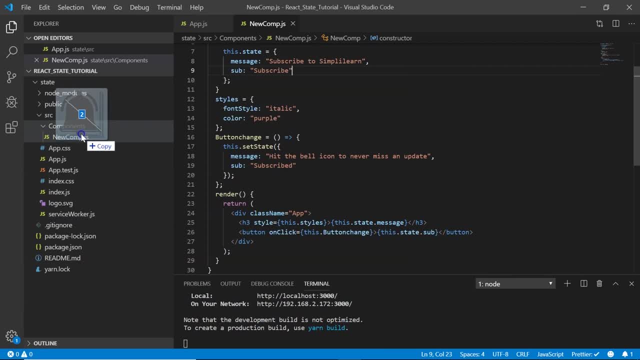 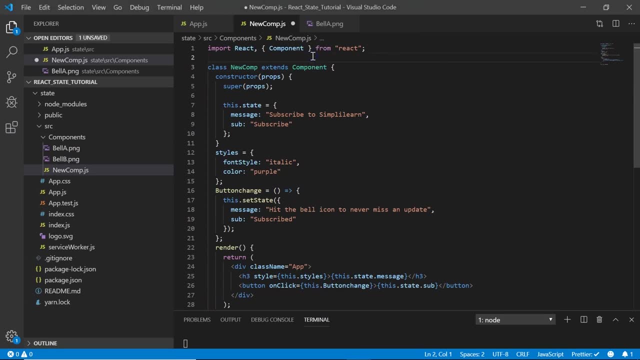 So I drag and drop both the images in my components folder. Alright, Now let's import these images into our newCompjs file. Here I say: import bellA from bellApng. And again I say import bellB from bellBpng. 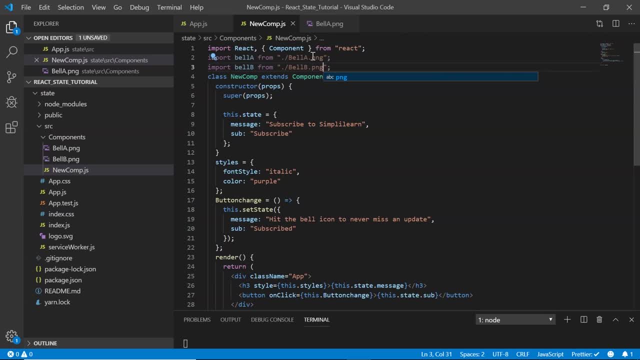 Everything is fine. Let me save it. To display the image on the screen, we make use of the image tag. Now, this tag has two attributes: One is the source attribute that specifies the URL, and the other is the alt attribute that specifies an alternate text for the image. 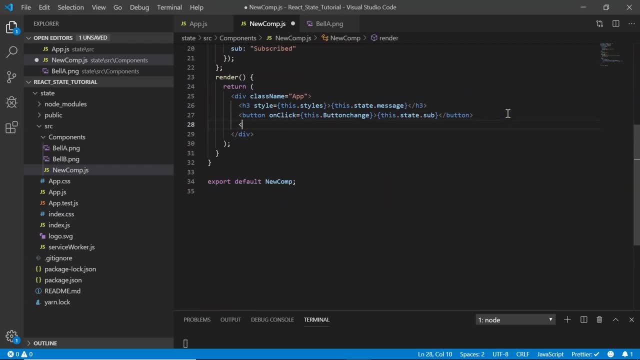 So here in my component I say I make use of a paragraph tag that will help display the image in the next line, and then I use the image tag. Now, since my image changes once it's clicked, I have to define a property and pass the event. 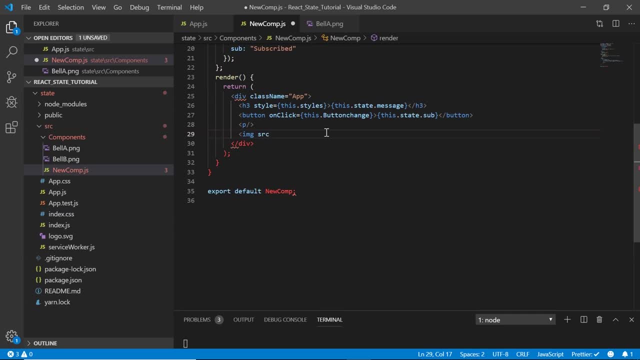 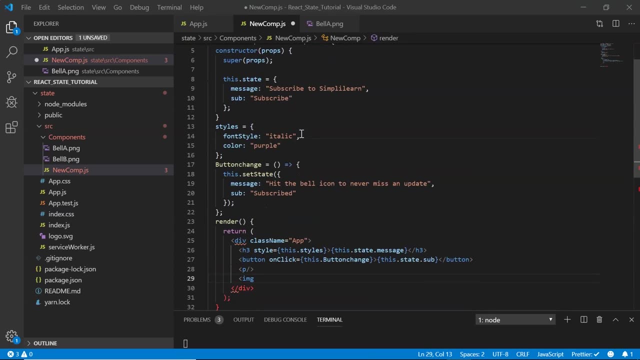 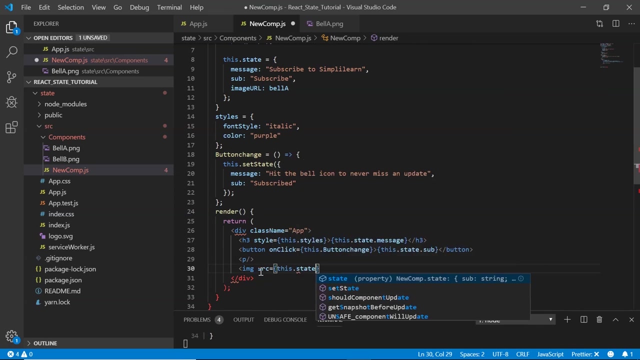 handler click that will update the image. So here, before specifying the source, let's go back to our state and define another property, that is image URL, and let's set it to bell A. since that is the image that I want to display, first, Let me save it, and here in my image tag I say: source equals thisstate. 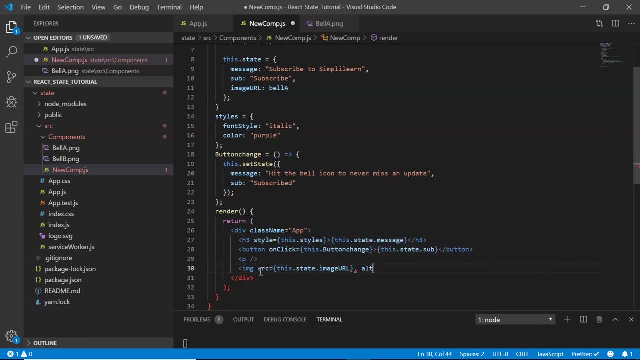 image URL. and then we have the alt tag, and I do not want to display any message, so I leave it as it is. Now let's save it, and if you look at the browser, we have a bell displayed. However, now let's change the dimensions of the bell. 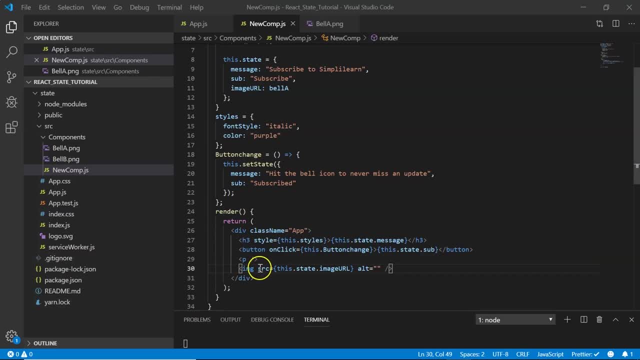 I do not want such a huge bell. So back in my VS Code I define style with width, say, 30 pixels, and a height with again 30 pixels. Let me save this. And now, if you look at the browser, We have a smaller icon. 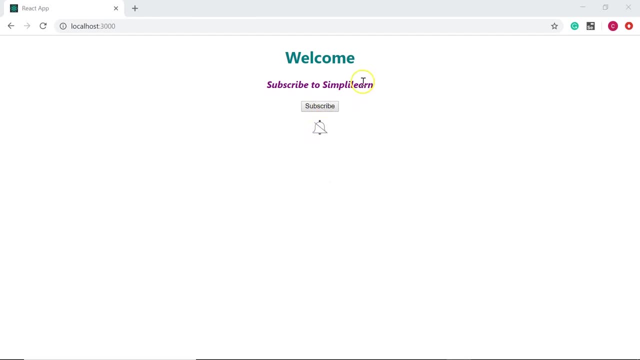 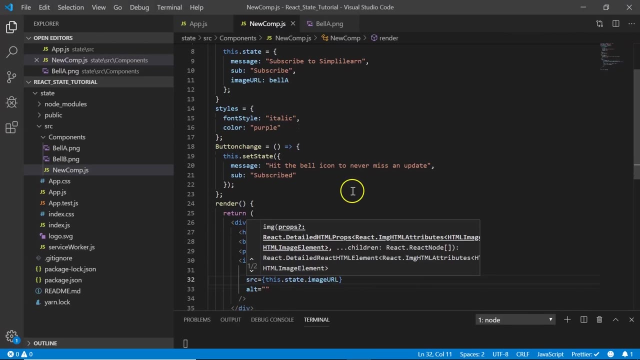 So once the user clicks on this image, the image changes and the message displayed here gets updated. To do that we'll have to define an event. So let's go back to our VS Code and here in my image tag, let's say onClick and define. 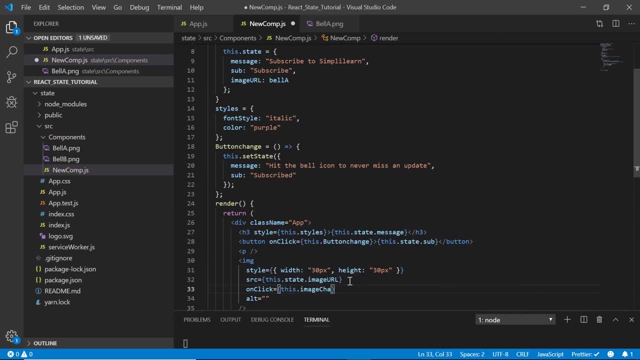 a method, say thisimageChange. and now we define this method here. I say imageChange and make use of an arrow function. again and again I use the setState method. I update the image So I say imageUrl is now set to bellB and the message is updated to: thank you happy. 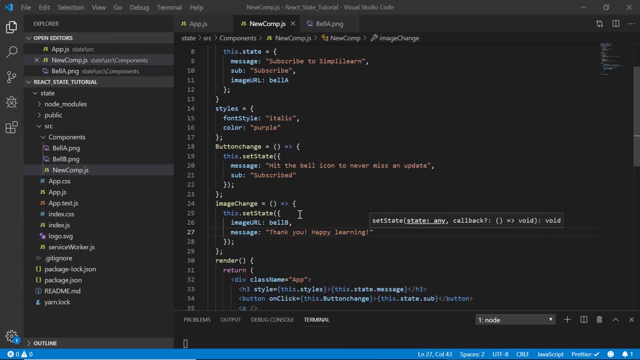 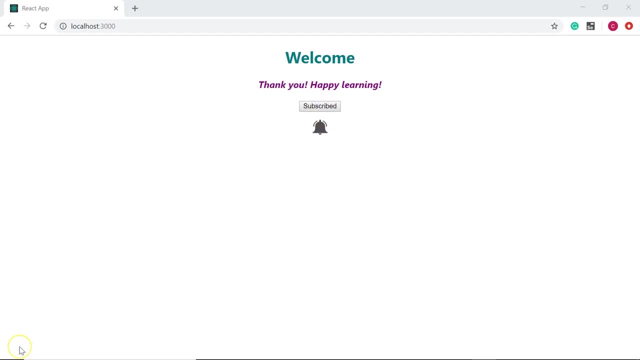 learning. So let's save this now. and if we look at the browser, we see the image and once clicked on it, the image gets updated and the message changes. So, finally, let me refresh the browser once and show the full execution. Let me refresh. 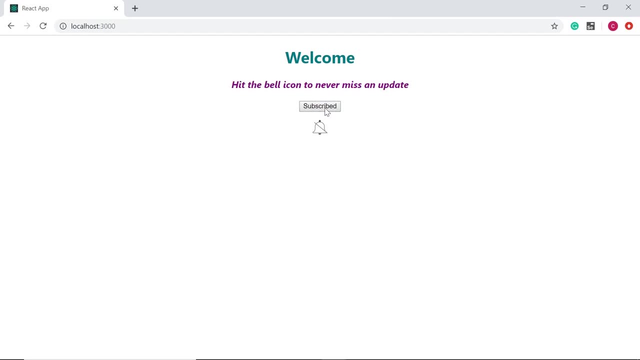 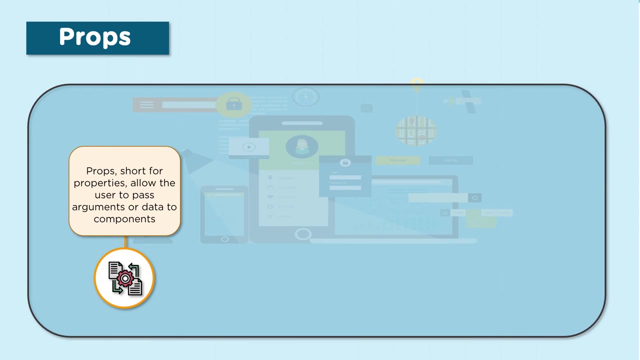 Following the instructions, Let's click on the subscribe button, Let's go back to our VS Code And now it says: hit the bell icon and once I do that, the image updates and the message changes. Props- short for properties- allow the user to pass arguments or data to components. 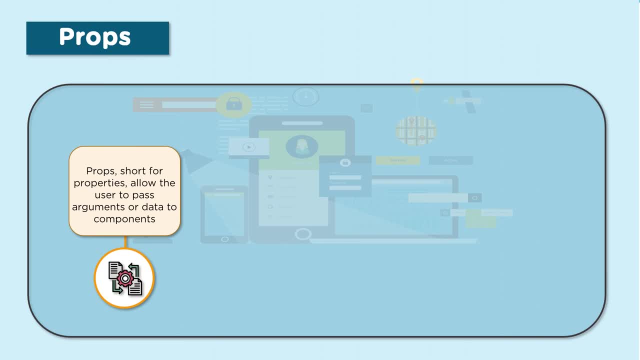 A parent component can pass additional information to its children using props. Properties help make components more dynamic. Props are passed to components in the way similar to that of HTML track attributes. Now we'll look at this a little later in the video. Props in a component are read-only and cannot be read. 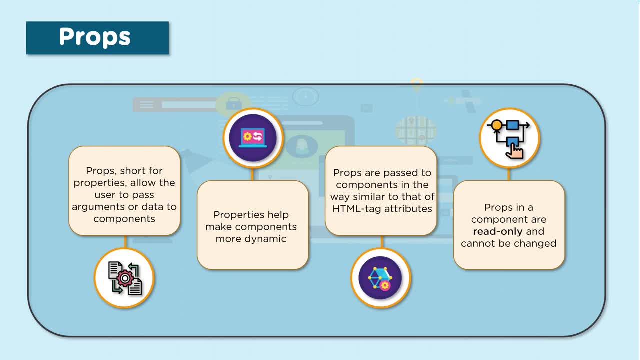 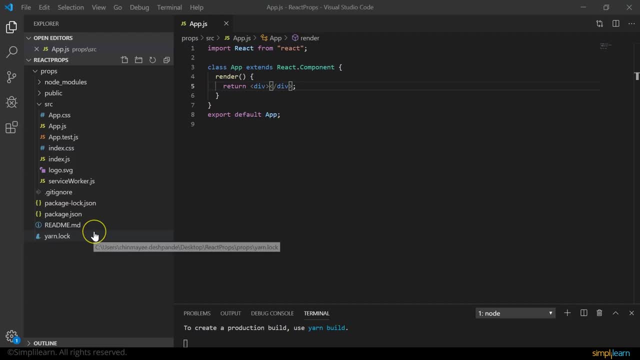 One thing to remember is that props are sent by the parent to the children components. Hence, the children components cannot make any changes to these props. Now that we've learnt about props in brief, let's go ahead and create our application using props. 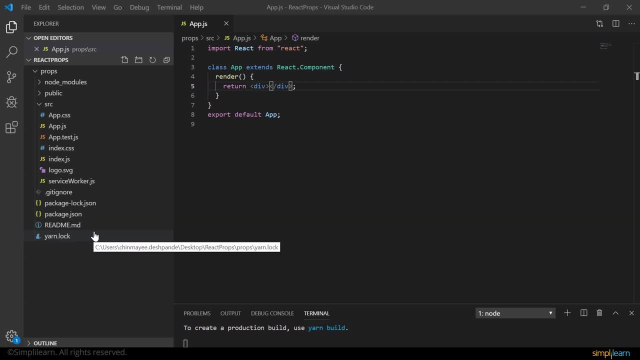 If you're new to this tutorial, I suggest you go to the React installation and react components video on our channel. So back in my code editor, that is, VS Code, I've opened a folder called react-props and now I'm going to create a component. 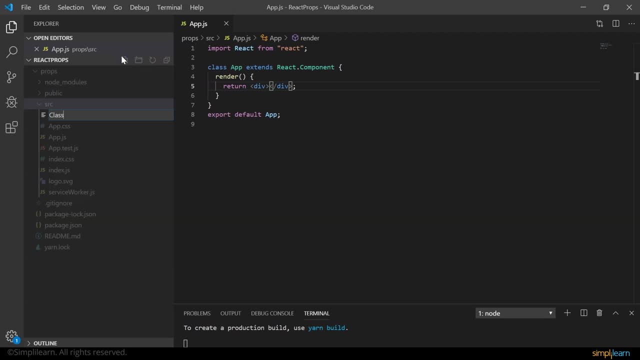 I'm going to create a component, A class component, and I'll call it class-propsjs. So let's create the class component. I give rce the snippet and here I display a message saying an h1 tag, basically Alright, Now let me get rid of export here and import it in my appjs main component. 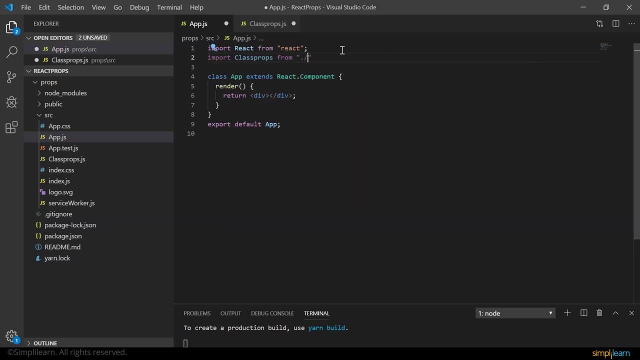 Here I say: import class-propsjs. Alright, Now we define the class component in our render method. let's say: alright. Now, if we go back to the browser, you see hello learners, welcome to Simply Learn. Now let's say we want to individually welcome every student. 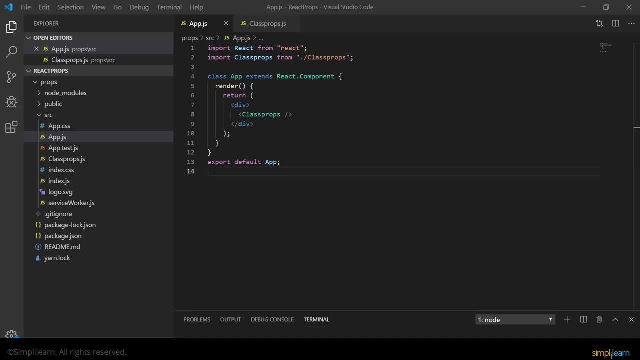 Instead of retyping the message for everybody, we can pass their names as props. Now let's see how to do that. Now we pass the name as a property from the main component, that is, appjs, To the child component and render this onto the browser. 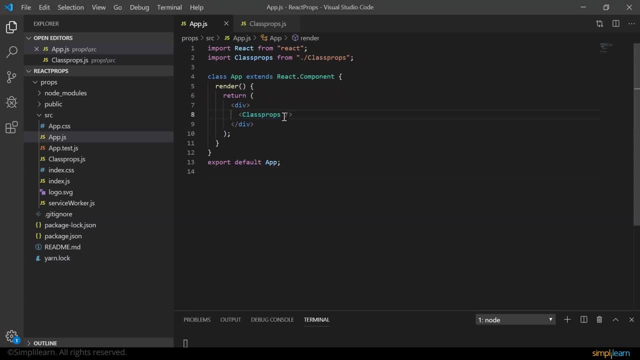 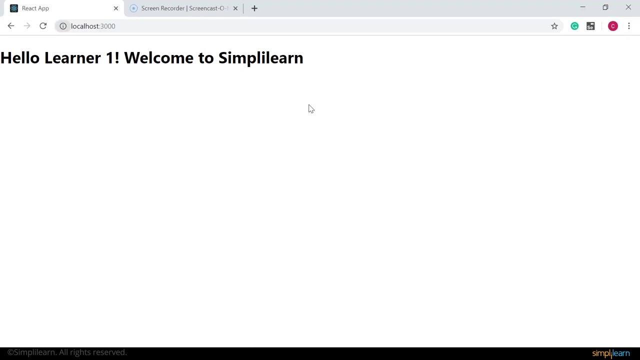 So let's do that. So here, while I'm defining my child component, I say name, I save it. and here in my child component, instead of learners, I say I use a keyword: thispropsname. Let me save it. and if you look at the browser, we'll have: hello, learner 1, welcome to Simply. 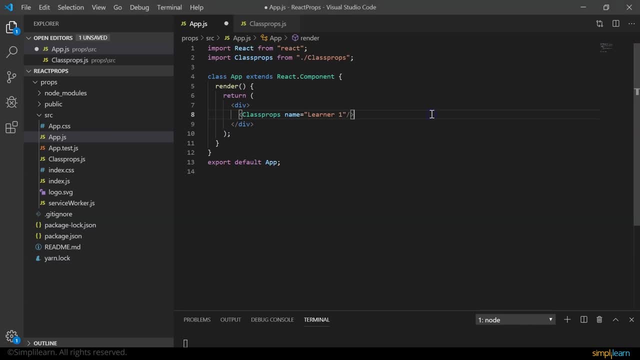 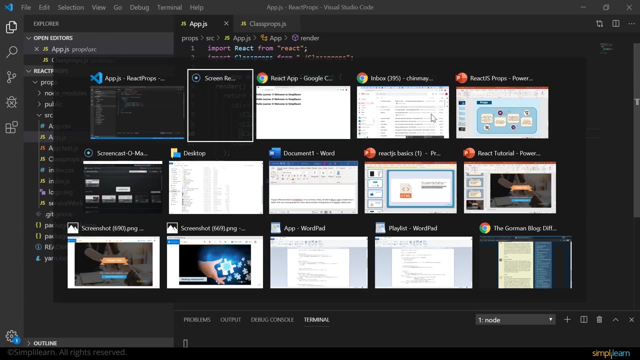 Learn. Now let's go ahead and welcome learner 2 and learner 3.. So I again say: class-props name equals learner 2.. Alright, so if we save and look at the browser, we'll have all the three learners displayed on the browser. 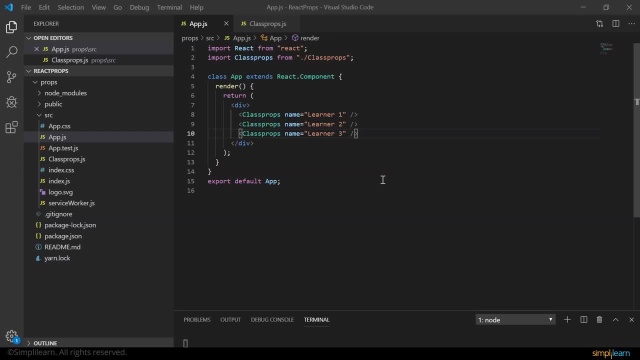 We can also pass multiple props to the child component. Now say, for example: we want to welcome the student from a particular place, So we say welcome learner 1 from place x. So I can here define another property, say place and say place similarly. 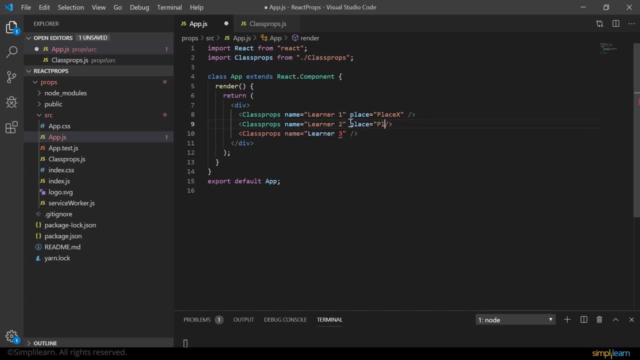 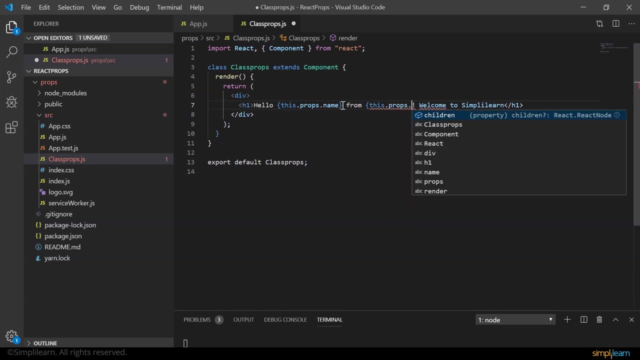 I can do it for the rest too. say: place y. Now let's go back to our class-propsjs component and here say: hello, learner 1 from thisprops. Okay, Okay, So now we have our class-propsjs component. 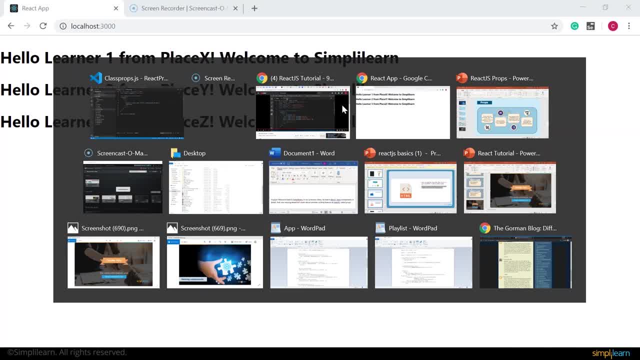 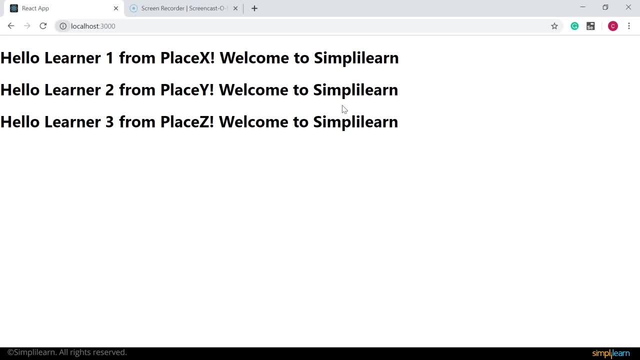 Let me save it. and if you look at the browser, now we have hello learner 1 from place x, place y and place z. We can also display whatever we want between the opening and closing tags when invoking a component. Now this is facilitated using propschildren reserved keyword. 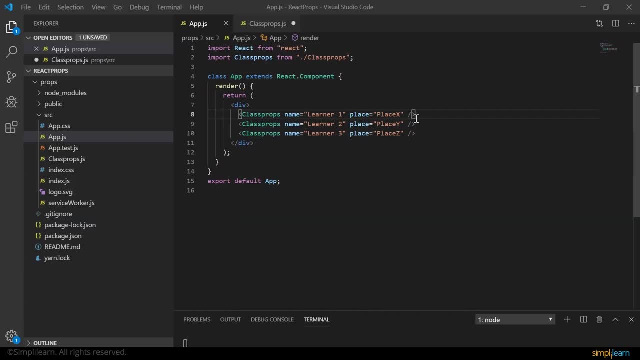 Now let me explain to you how it's done with an example. Here let's split the self and closing tag into an opening and a closing tag and in between them. So here I have a message within the paragraph tag: let me save. and in my child component. 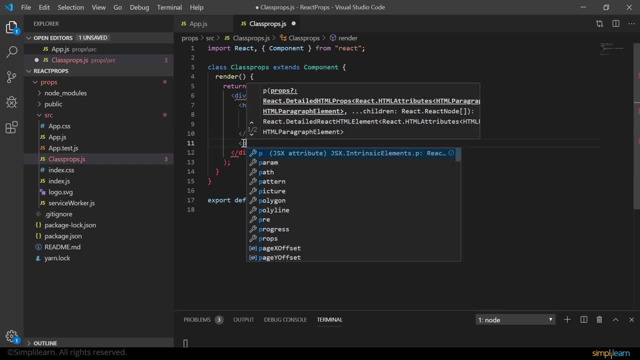 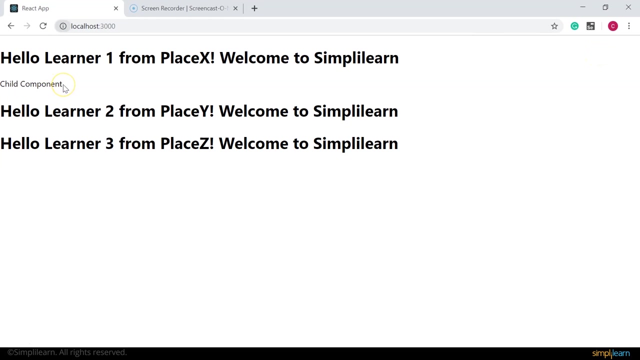 after my h1 tag, let me use a paragraph tag, and here let's use the reserved keyword thispropschildren. So let's save it. and now, if you look at the browser, you can here see the message displayed: child component. So propschildren can be used. 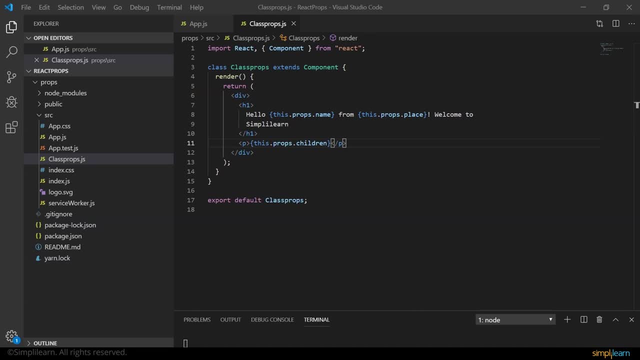 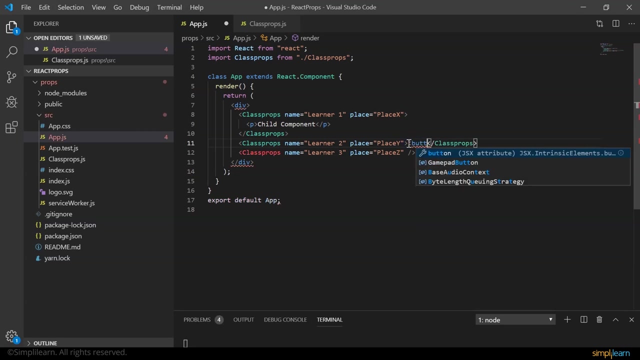 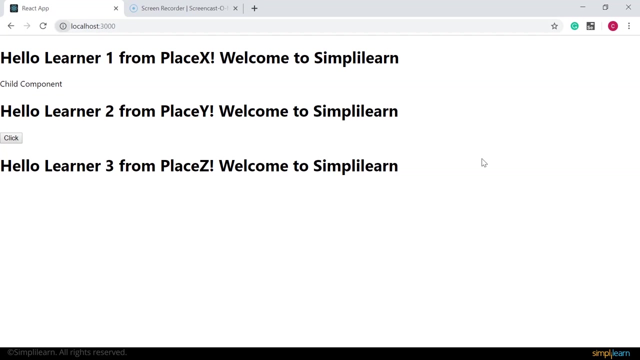 When components do not know about their children ahead of time. This is commonly seen in components like sidebar and dialogue that represent generic boxes. So let's go ahead and create a button tag and check again. So here I'll split it and add a button tag and say click and let's check our browser. 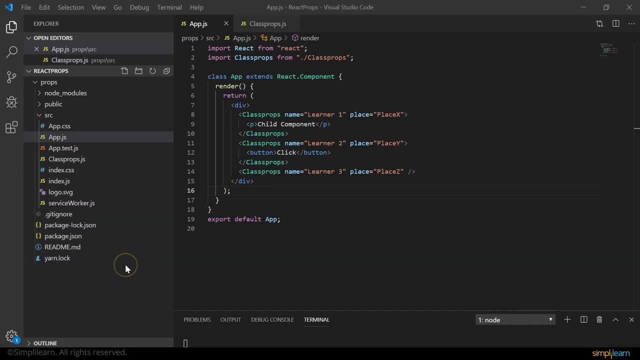 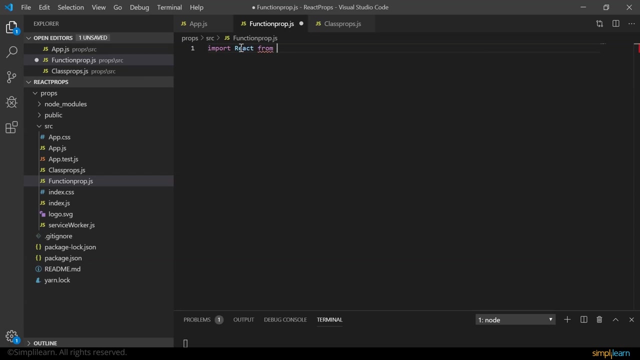 Here we go, We get the output as expected. All right. We saw the usage of propschildrenchildren For class components. Similarly we can use it for functional components. So let's go ahead and create a functional component. Let me call it. I say import, react from react, and then I say function, function, props and 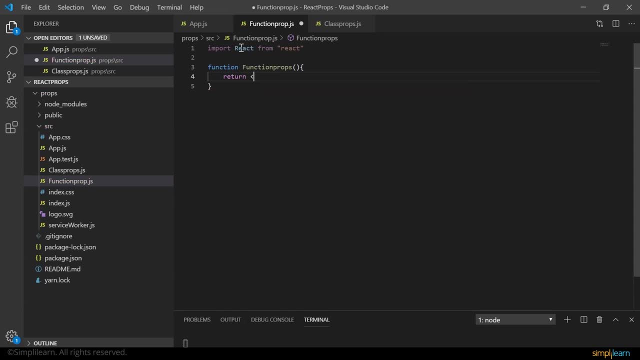 here I return an h3 tag. I'll say: this is functional component. And here I return an h3 tag. And here I return an h3 tag. I'll return another h3 tag saying hello learner. So let me save this and let's export it.